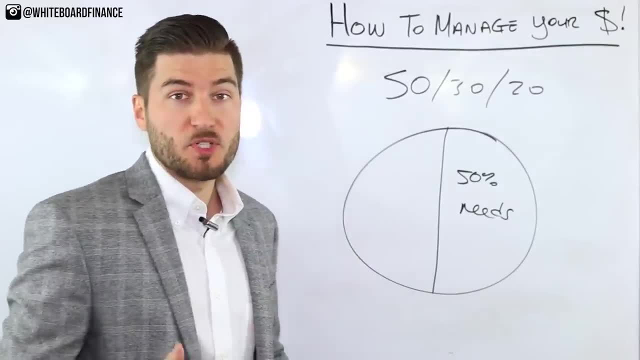 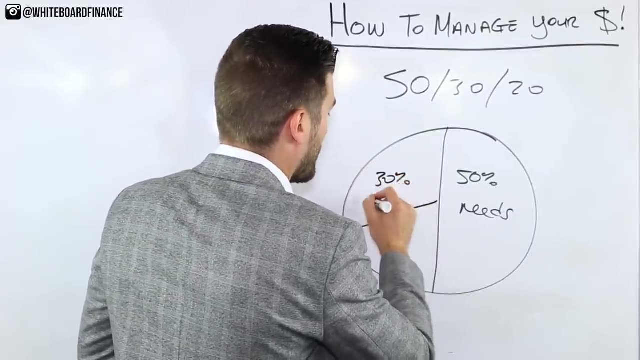 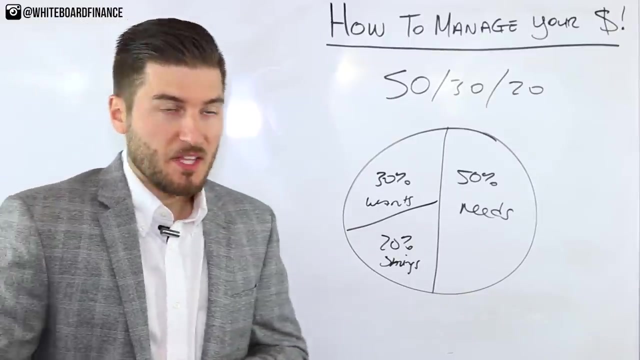 your money is going and an ideal personal budget portfolio. So 50% are needs, let's call this- 30% are going to wants and then 20% is going to savings or paying off debt. So now that you have a visual representation, let's break down each one of these numbers. 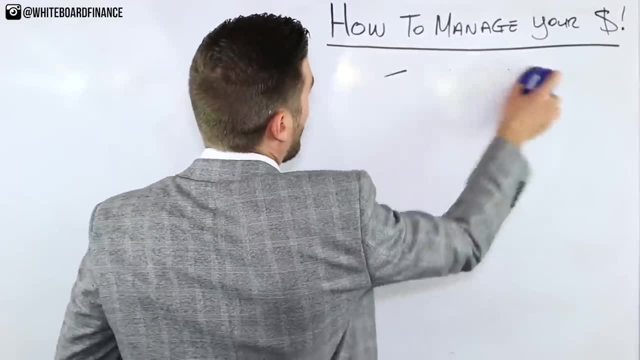 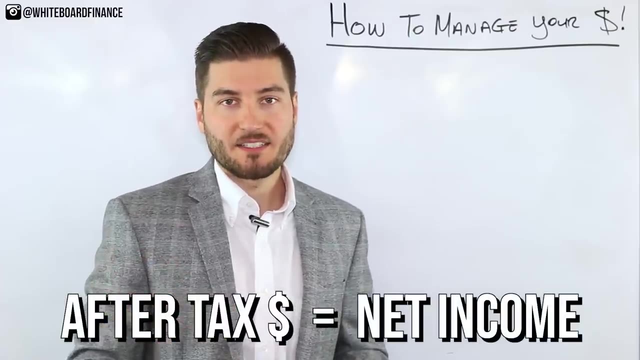 and give you examples of each, so that you can be gauging your own personal finance based on these metrics. Keep in mind we're working with after-tax dollars, which is called net income, So you may have a gross pay of, let's say, 50 grand a year. 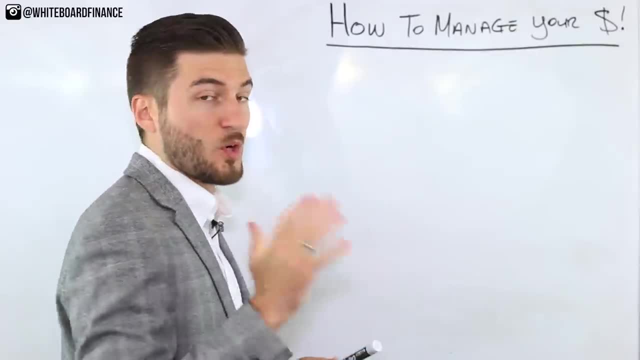 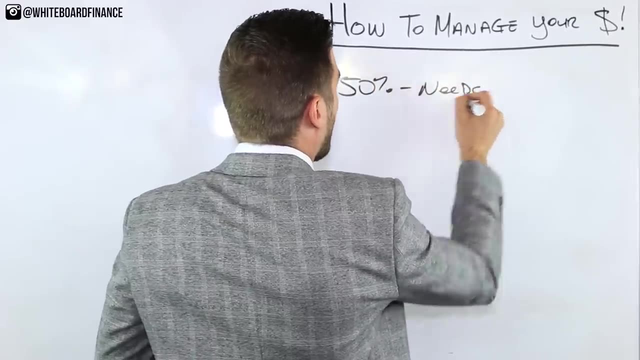 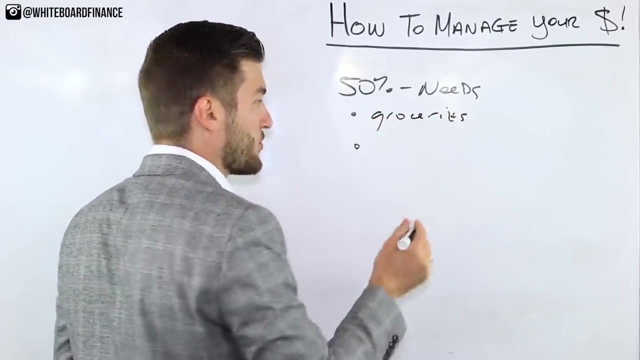 but after tax is. you're only dealing with another specific number. We're using that after tax dollar number. So, in terms of the 50% needs, what are some things that can be included in this? So let's think about regular living expenses. So we have groceries, we have housing, whether you have a 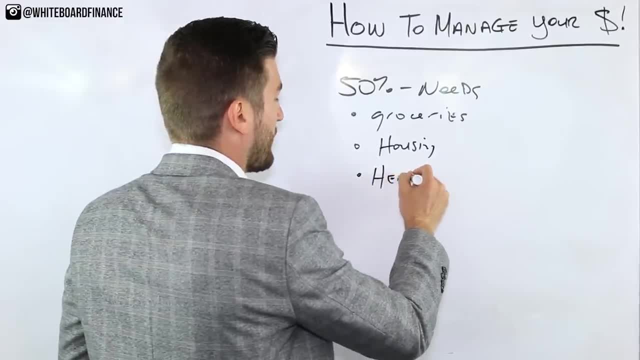 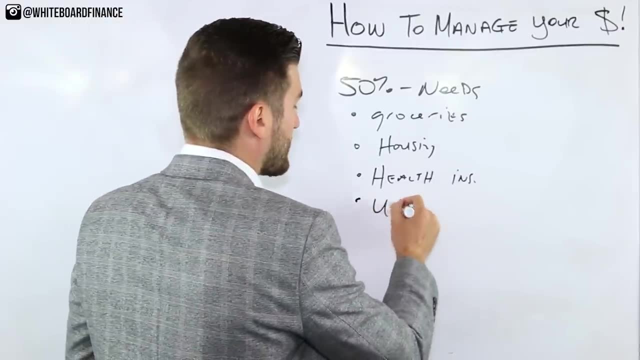 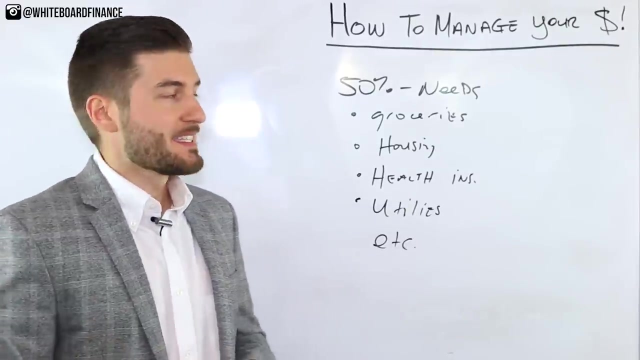 mortgage or rent. you have insurance for health. Heaven forbid something happened to you. I would consider health insurance definitely a need. You can have utilities, so electricity, things like that, etc. etc. So the way I define a need is that it's basically something that would greatly. 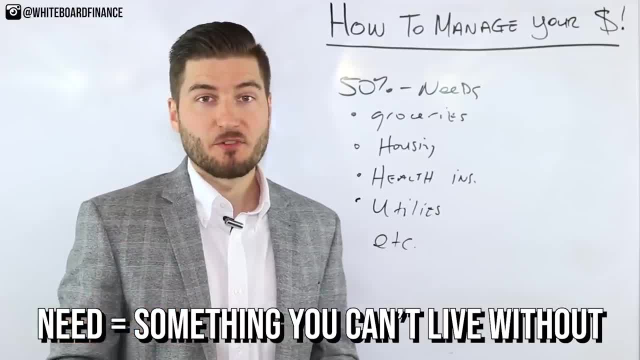 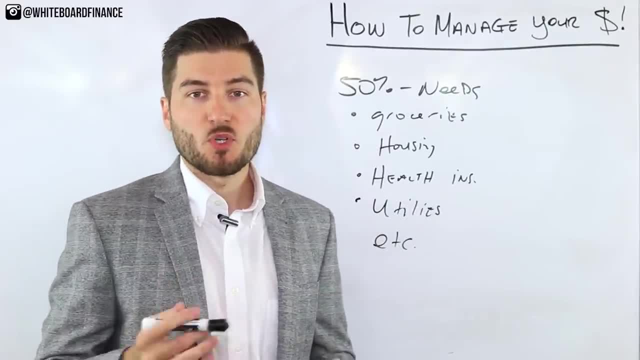 inconvenience you or something that you literally cannot live without, So food, shelter, things like that. So when you budget 50% towards your needs, remember that those are what you're looking at. So the next logical area to go into is going to be: 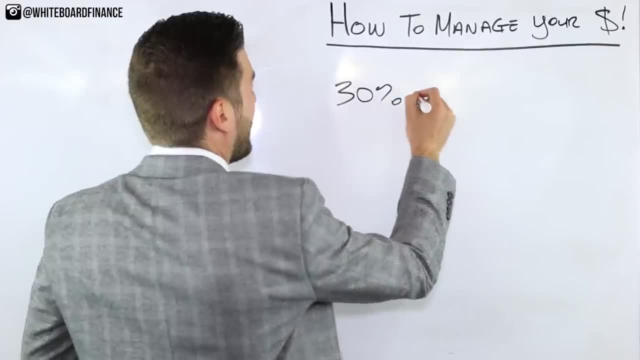 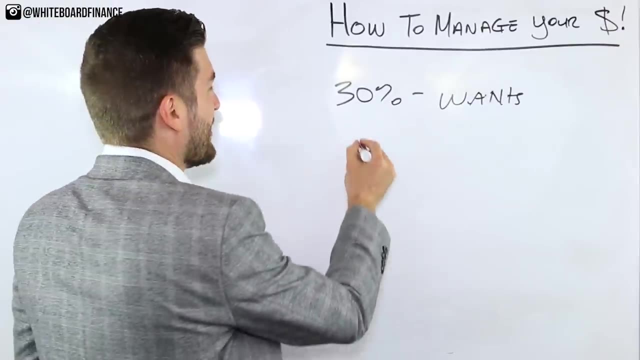 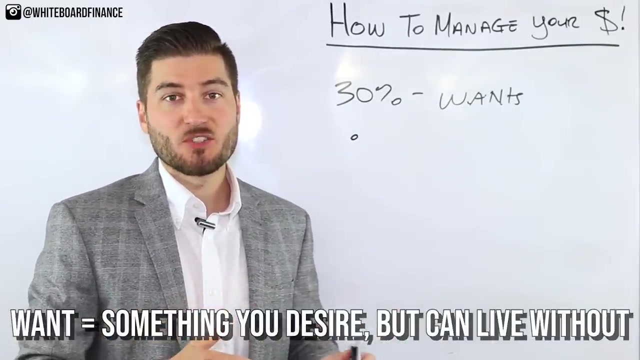 what is really considered a want, And I think this is where most Americans run into the difference between wants and needs. So a want is something that causes a minor inconvenience in your life. It's not necessarily a need to where, hey, if I don't eat or if I. 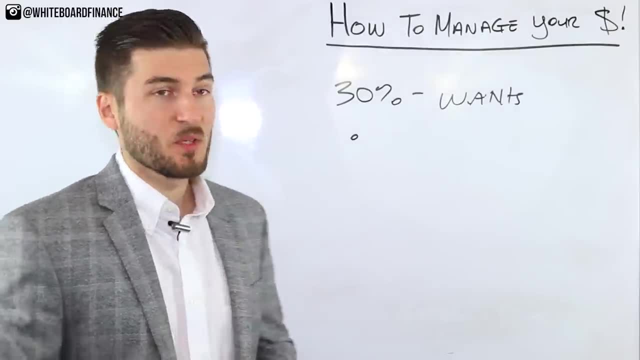 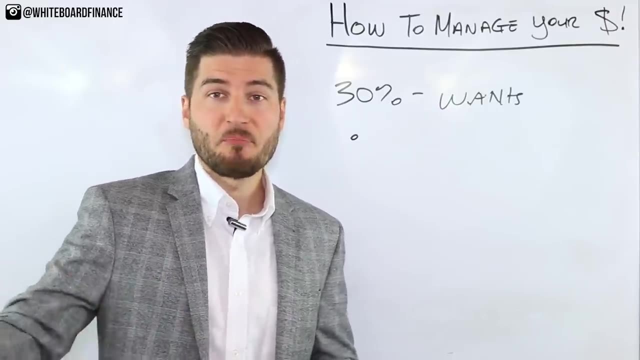 don't have shelter, I may die. A want is something where it's like, hey, am I willing to give a minor inconvenience, like dropping Netflix or not having Hulu or not buying a brand new grill to grill a steak on. You know those are needs. OK. so some of the 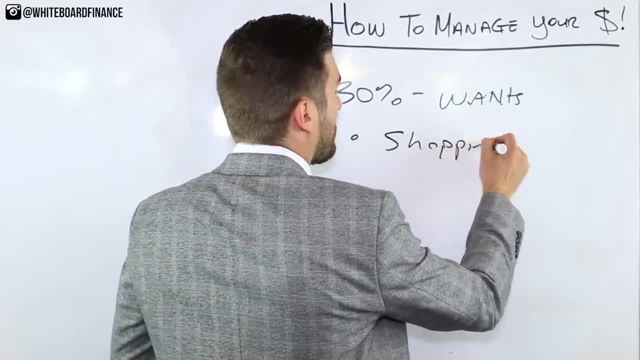 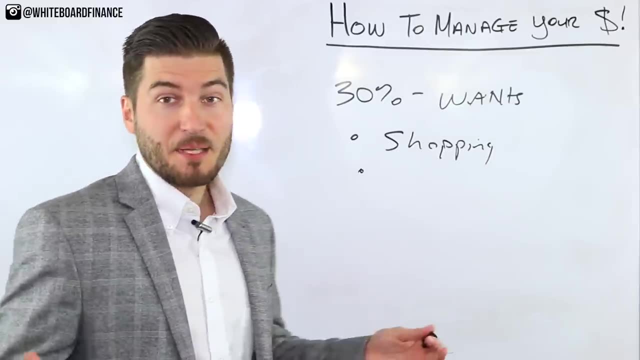 things that would fall under this category would be things like shopping. You absolutely need to shop for brand new clothes, right? this second: Are you going to drop dead if you don't get a new pair of shoes? Maybe my wife will, but I know that I can survive. you know dining out, I think this. 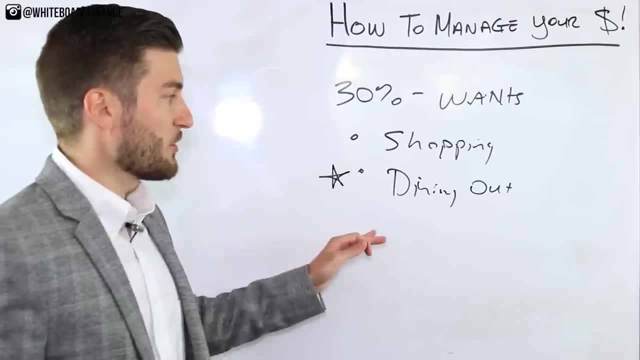 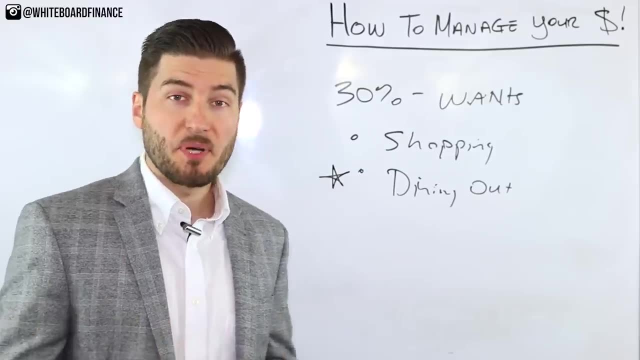 is a big one for Americans. A lot of people, for whatever reason, their lifestyles are so busy that you know it's easier just to jump in the car and go grab something to eat rather than preparing the food yourself, Hobbies. So I think that everyone should. 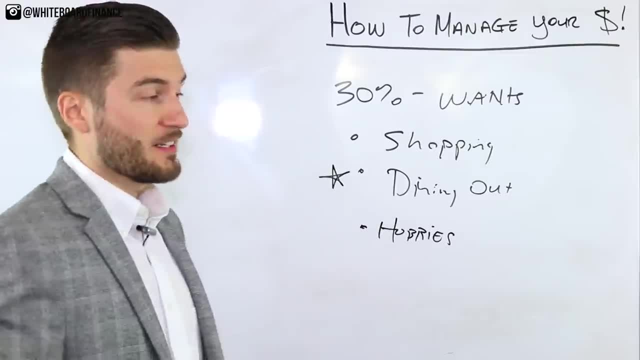 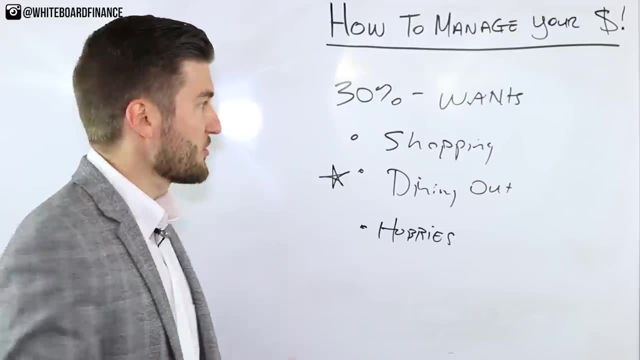 definitely have a hobby. That's one of the greatest joys of life. whether it's gardening, you know, you fly drones, you're a video editor, whatever you want to do, whatever it keeps you happy as a hobby, This definitely falls under a want, because it's not necessary to live. So again, guys, a want is. 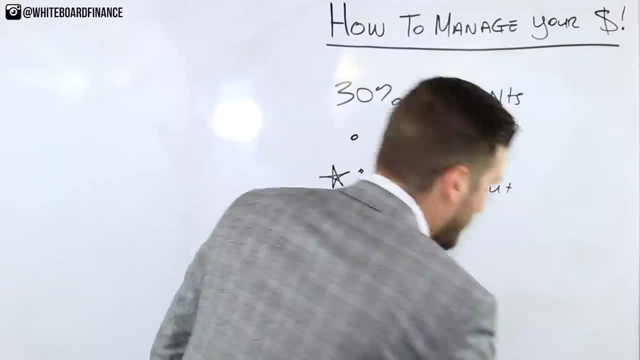 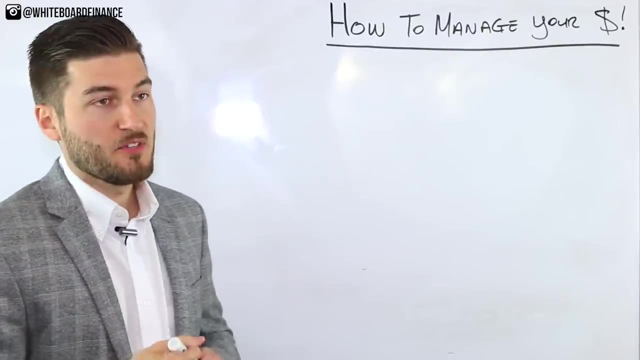 something that you don't necessarily need, but it improves the quality of your life greatly. So let's go to the last 20 percent, And I know a lot of this sounds basic, but until you actually write this down and understand where all your money is going to. 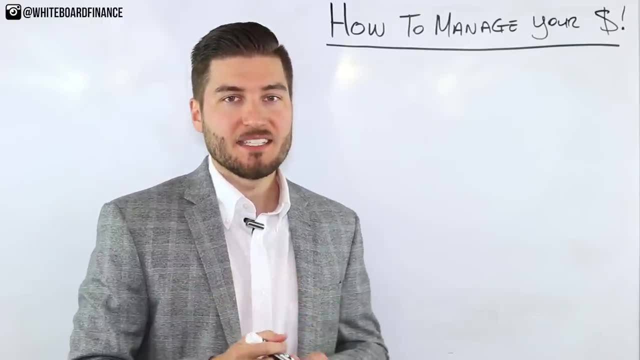 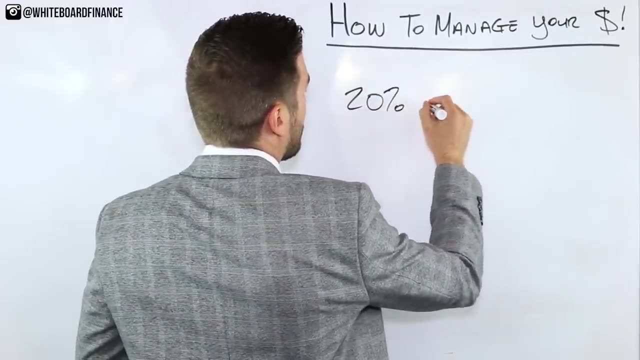 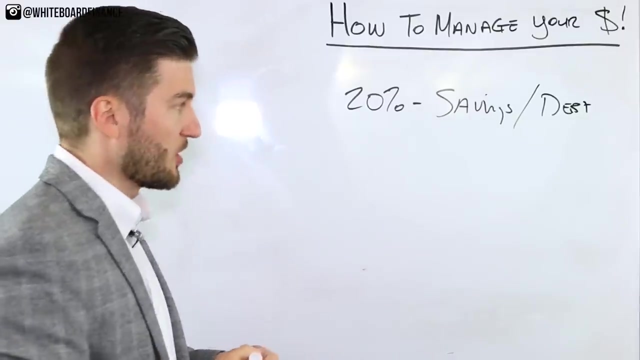 it's like your wants can easily creep into that needs category, to where they're both overflowing and you're in debt every month. So, speaking of debt, let's talk about savings. OK, so savings and paying off debt: This is where the last 20 percent of your income should go to, And again, 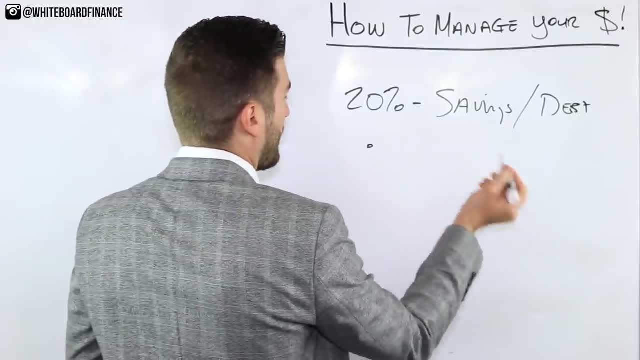 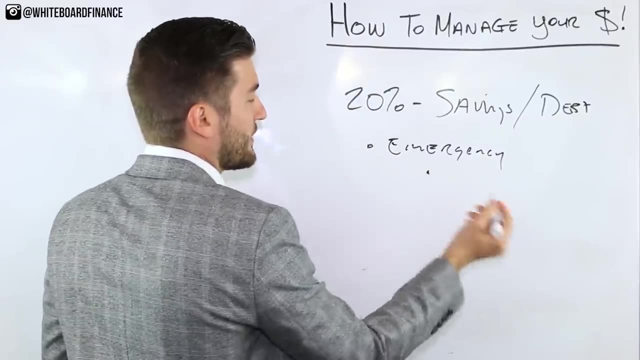 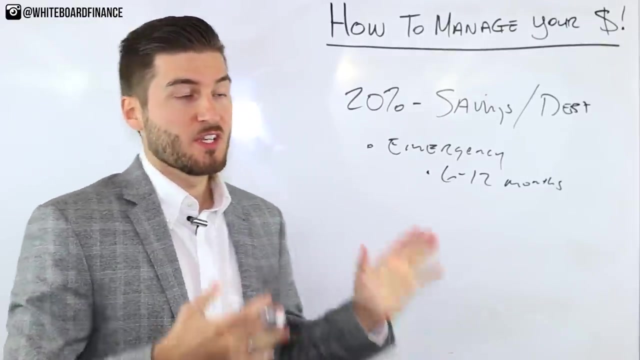 these are all net numbers. So if you have, let's call. let's say, for example, an emergency fund, OK, this I would consider savings. What I like to do for emergency funds this is six to 12 months of living expenses. So if you know that your needs category and a little bit of wants. 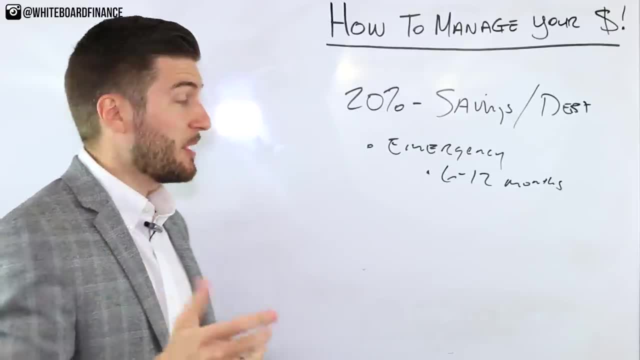 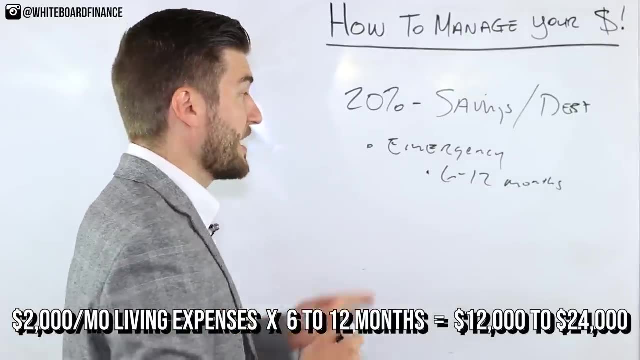 comes out to be, let's say, two thousand dollars a month for your entire family. you know that you need to save about twelve to twenty four thousand dollars in your emergency fund. I know that sounds like a lot of money, but you know one or two layoffs in a family of one or two income earners. 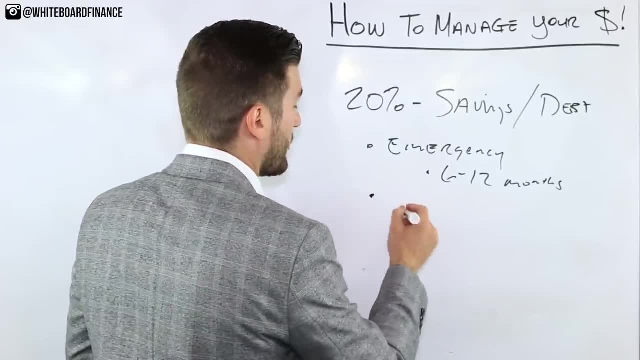 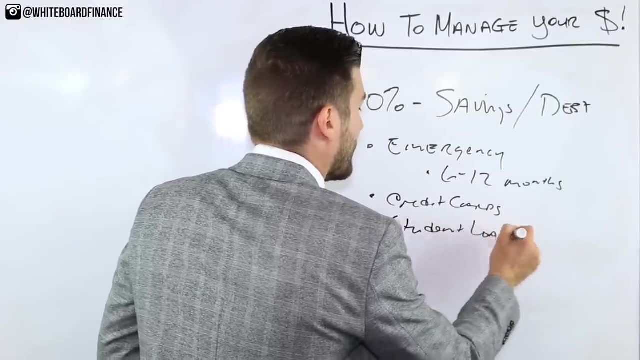 can really save your butt right there. You guys, obviously you know paying off debts. So if you have credit cards, you know student loans, things like that. These are debts that you should just smash using that 20 percent, And I will make another video about how to actually pay off debt.